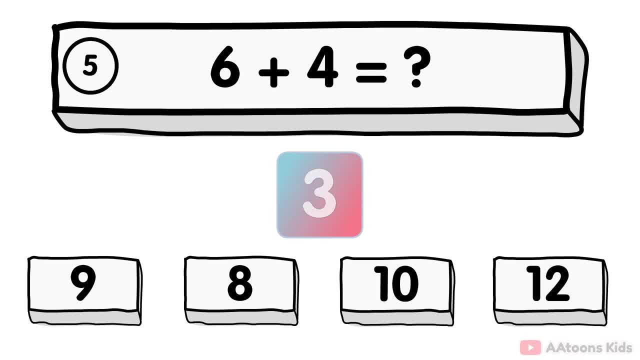 6 plus 4 is equal to 3.. What is 10? 10.? Please listen carefully: 10 is equal to 6.. In this quiz, we will remember 6 balls and 4 balls Now count together: 1,, 2,, 3,, 4,, 5,, 6,, 7,, 8,, 9 and 10.. 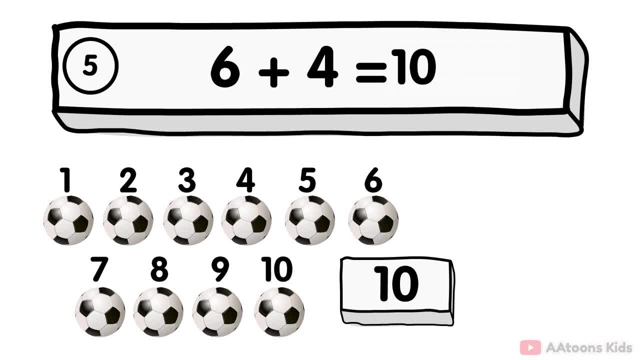 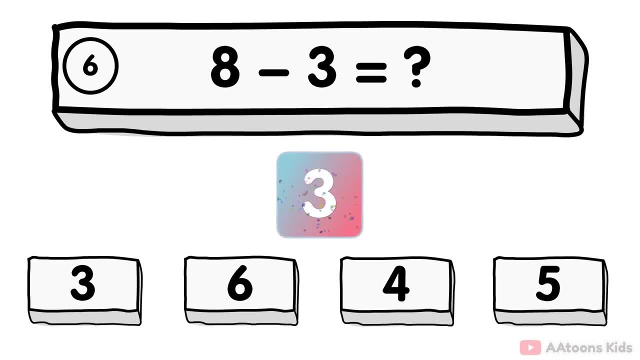 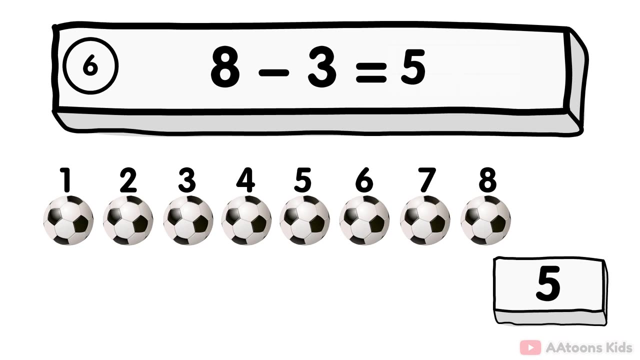 9 and 10. 9 and 10. 10. 8-3 is equal to 5.. Let's take the biggest number, 8, and subtract 3 from 8.. 1,, 2,, 3.. Now count the remaining box: 1,, 2,, 3,, 4,, 5.. So 8-3 is 5.. 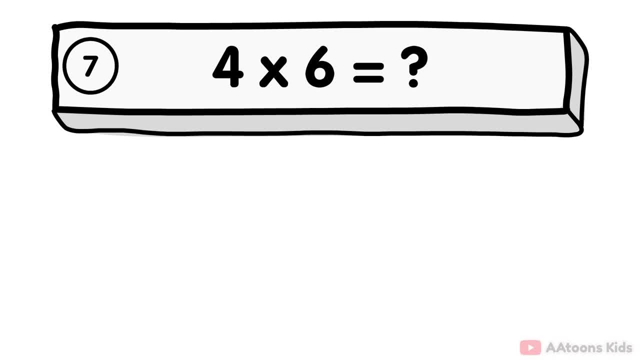 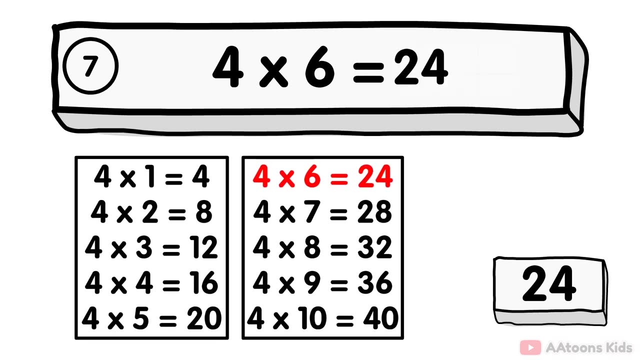 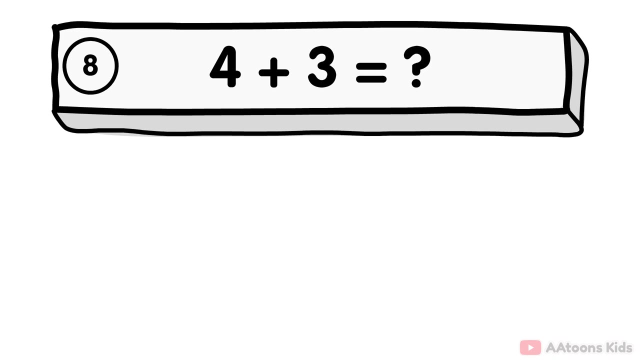 4 multiplied by 6 is equal to 24.. 4 multiplied by 6 is 24.. 4 plus 3 is equal to 7.. Let's take 4 balls and 3 balls. Now count together 1,, 2,, 3.. 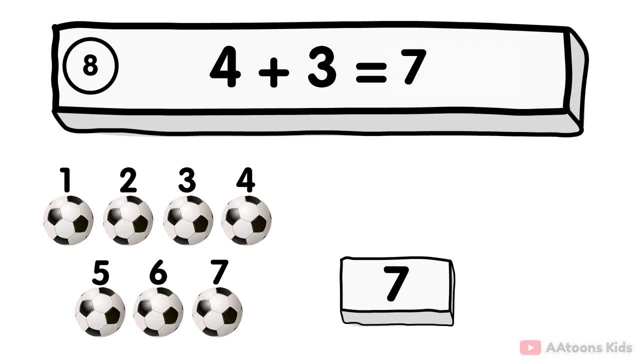 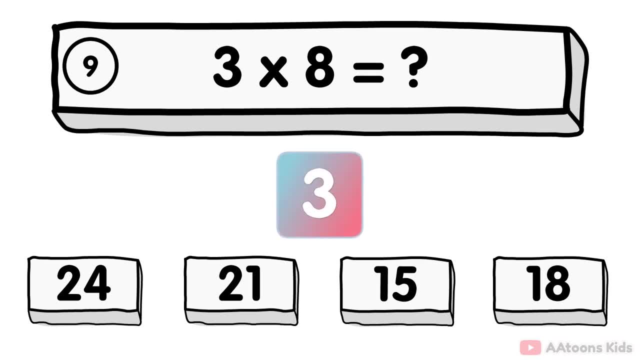 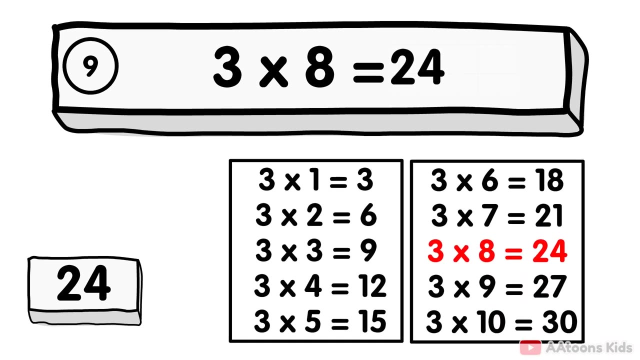 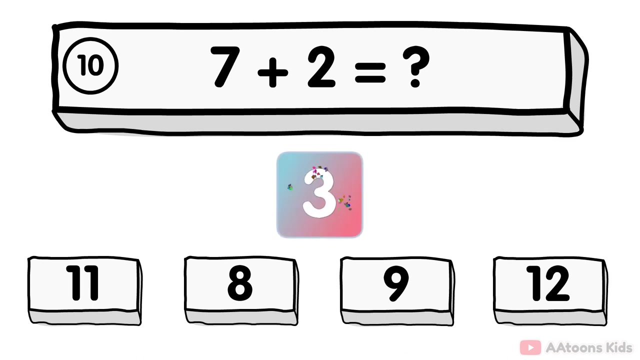 4, 5,, 6, 7.. 3 multiplied by 8 is equal to 24.. 3 multiplied by 8 is 24.. 7 plus 2 is equal to R้, 9.. Let's take 7 balls and 2 balls. 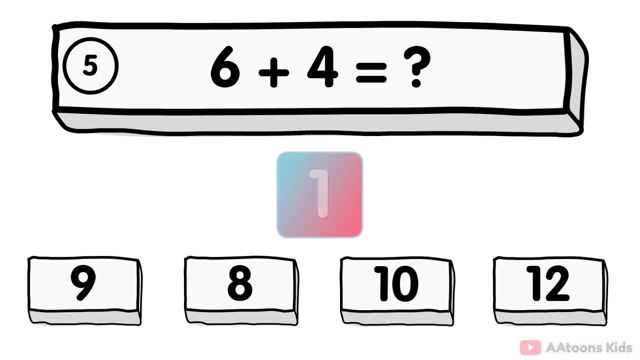 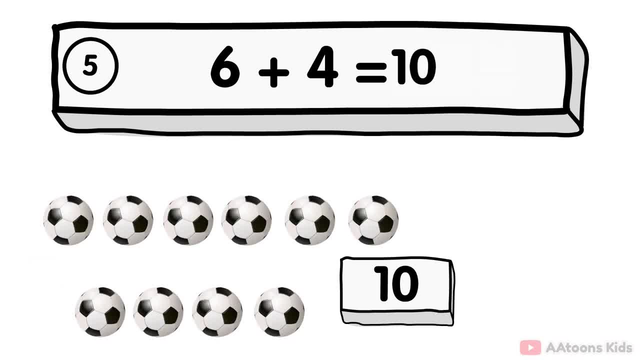 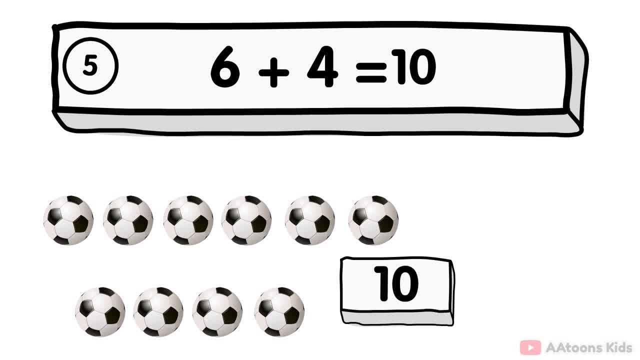 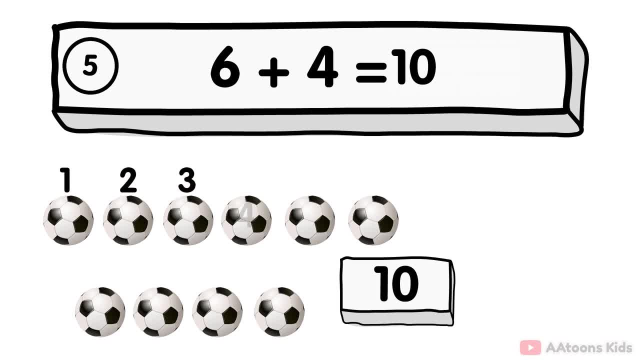 6 plus 4 is equal to 7.. 6 plus 4 is equal to 7.. 6 plus 4 is equal to 7.. 3,, 4,, 5,, 6,, 7,, 8,, 9, 10. 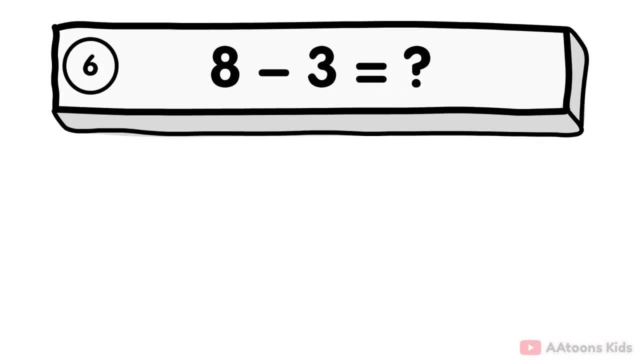 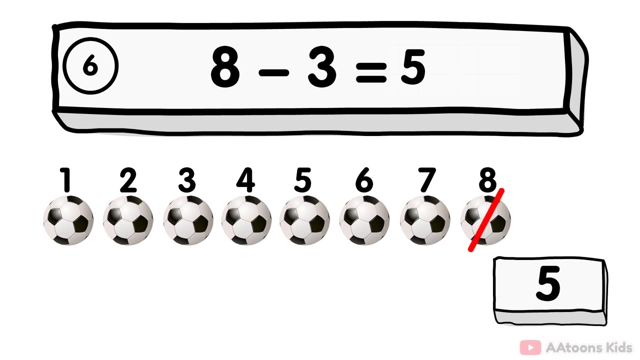 8 minus 3 is equal to 5. Let's take the biggest number, 8, and subtract 3 from 8. 1, 2, 3. Now count the remaining box: 1,, 2,, 3, 4, 5. 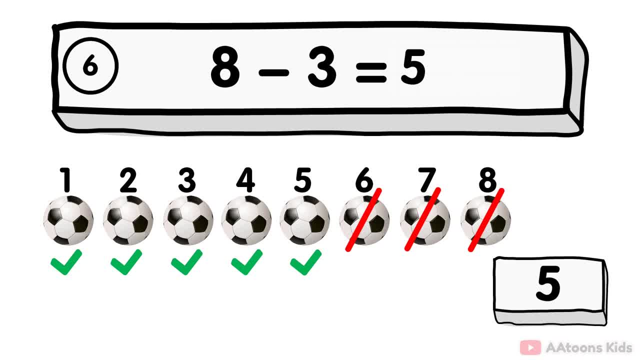 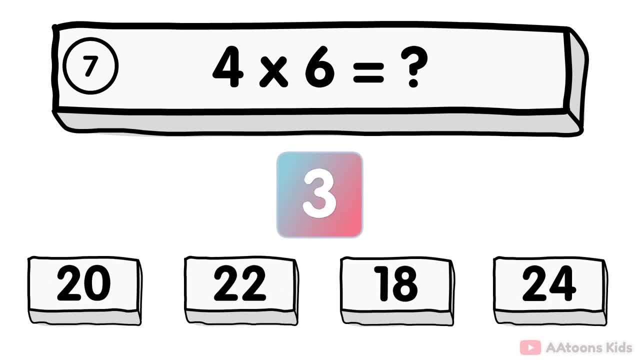 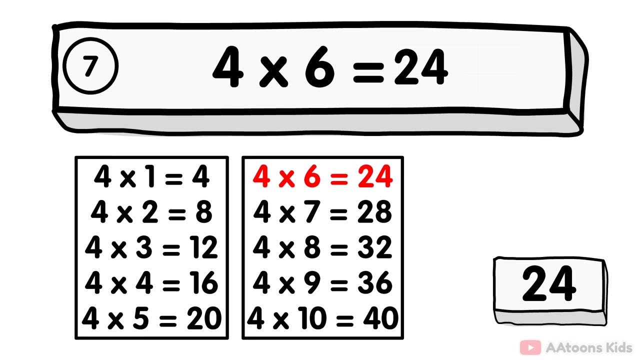 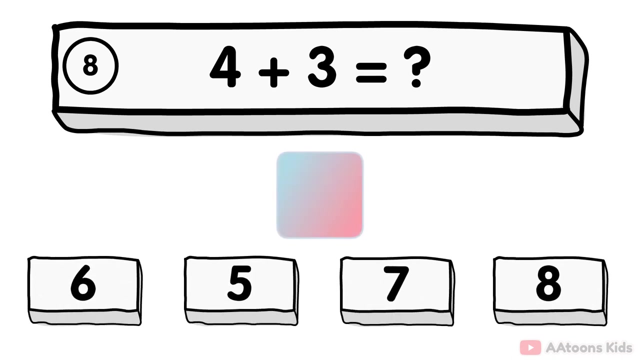 So 8 minus 3 is 5. 4 multiplied by 6 is equal to 24. 4 multiplied by 6 is 24. 4 plus 3 is equal to 7- 7. Let's take 4 bonds and 3 balls. 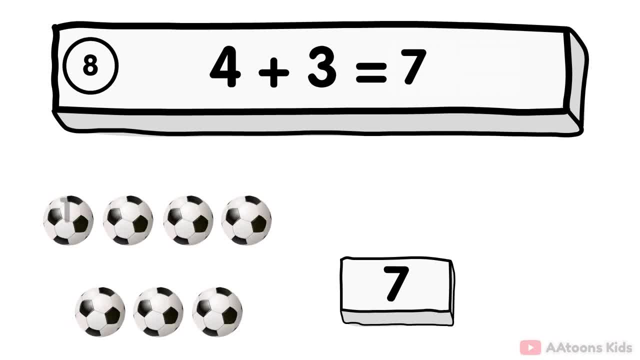 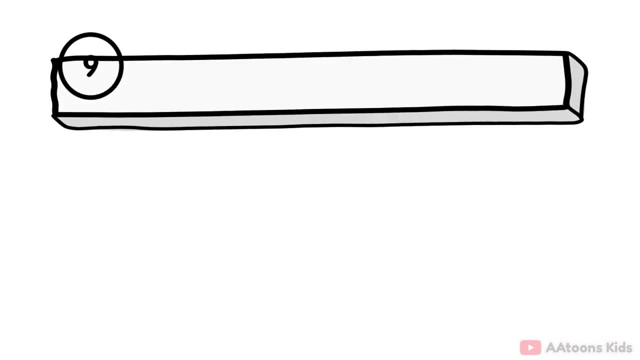 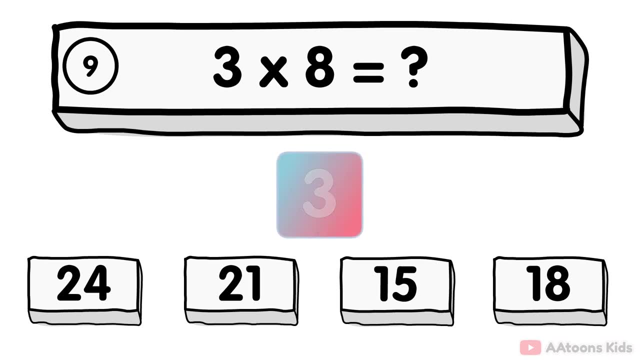 Now count together 1,, 2,, 3,, 4,, 5,, 6, 7. 3 multiplied by 8 is equal to 24. 3 multiplied by 8 is 24. 7 multiplied by 8 is 24. 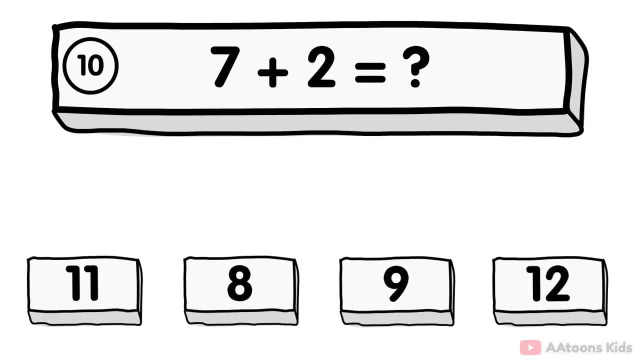 7 plus 2 is equal to 24. 7 plus 2 is equal to 24. 7 plus 2 is equal to 24, 24, 9. Let's take 7 balls and 2 balls. Let's take 7 balls and 2 balls. 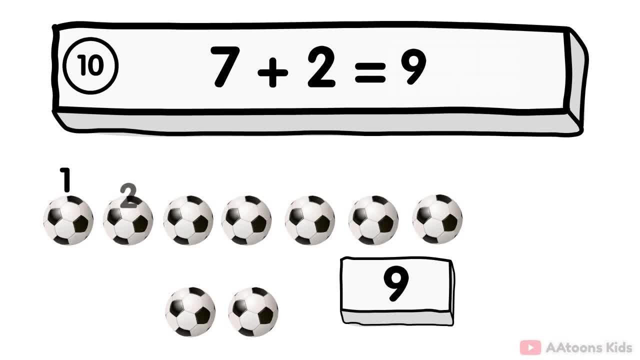 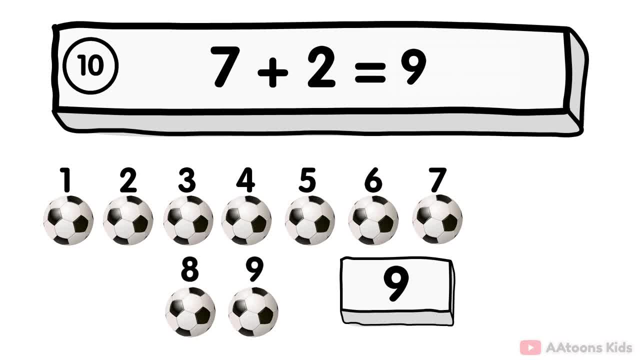 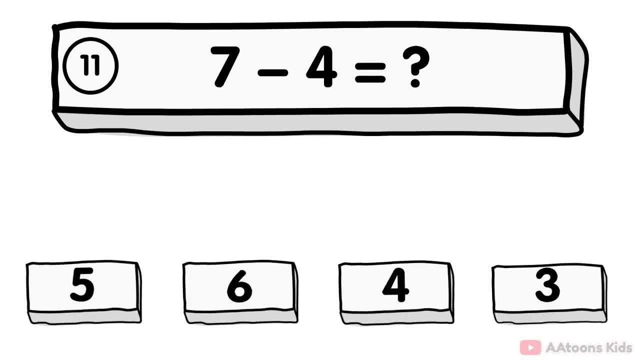 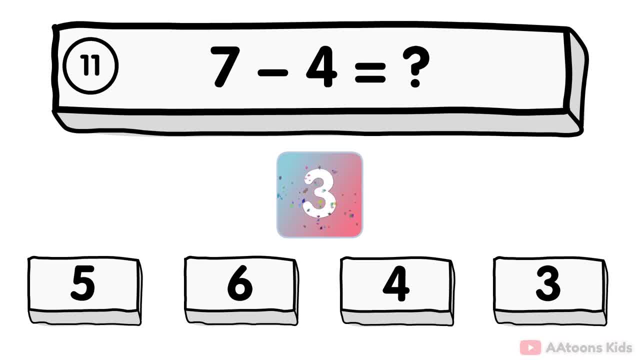 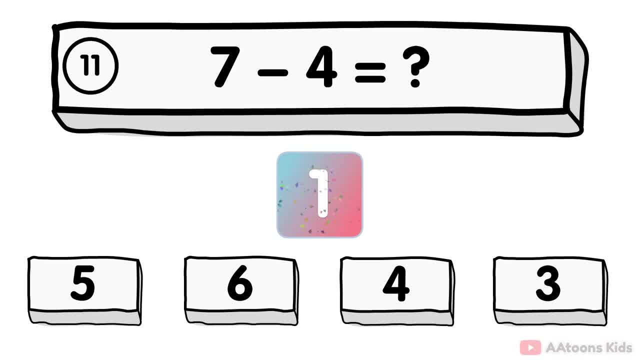 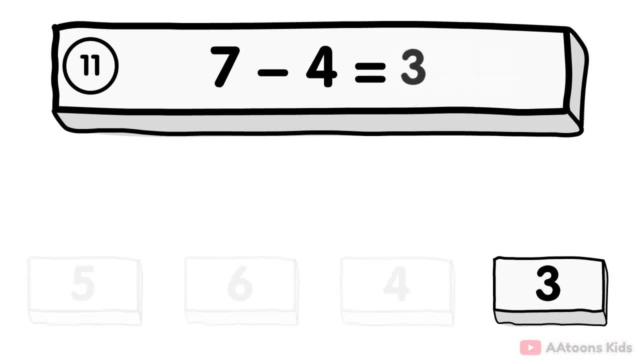 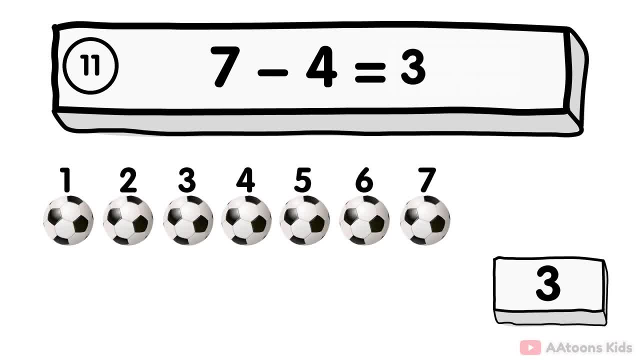 1,, 2,, 3,, 4,, 5,, 6,, 7,, 8,, 10, number 7 and subtract 4 from 7.. 1,, 2,, 3,, 4.. Now count the remaining box: 1,, 2,, 3.. So 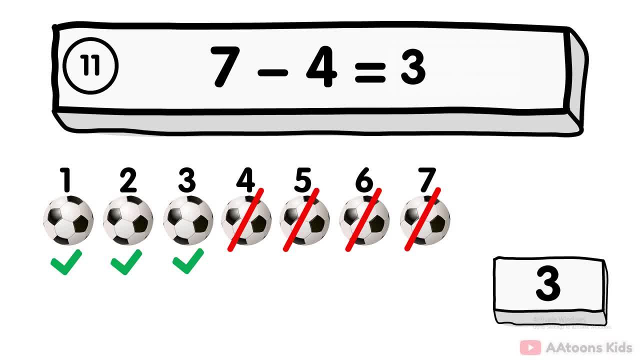 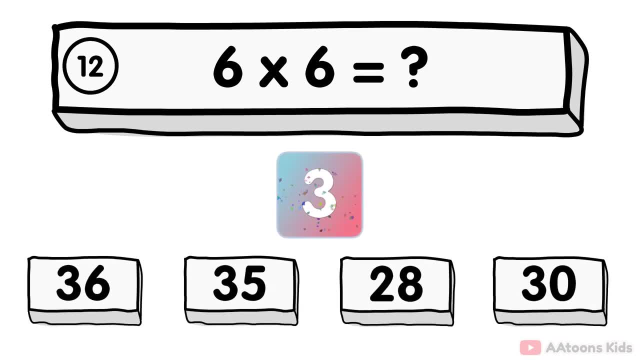 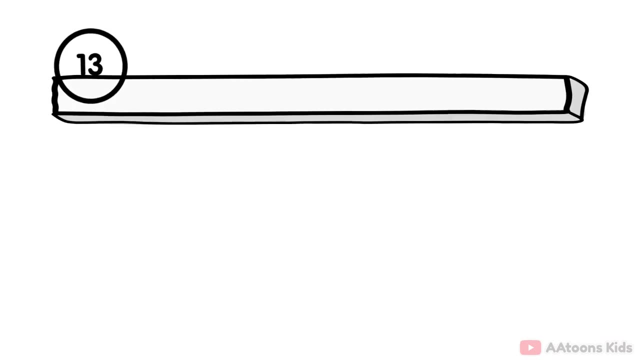 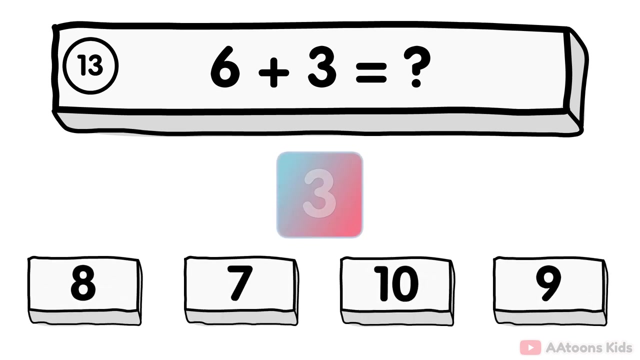 7 minus 4 is 3.. 6 multiplied by 6 is equal to 36.. 6 multiplied by 6 is 36.. 6 plus 3 is equal to 36.. So 6 multiplied by 6 is 2.. 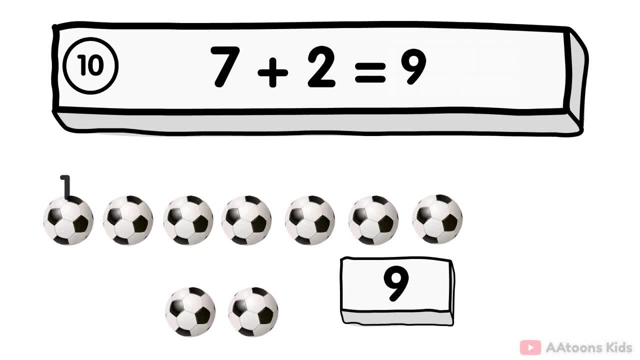 Now count together 1,, 2,, 3,, 4,, 5,, 6,, 7,, 8, 9.. 7 minus 4 is equal to 24.. 1,, 2,, 4,, 5,, 6,, 7,, 8,, 9.. 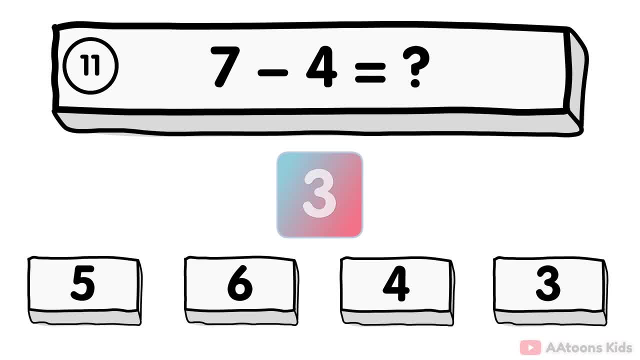 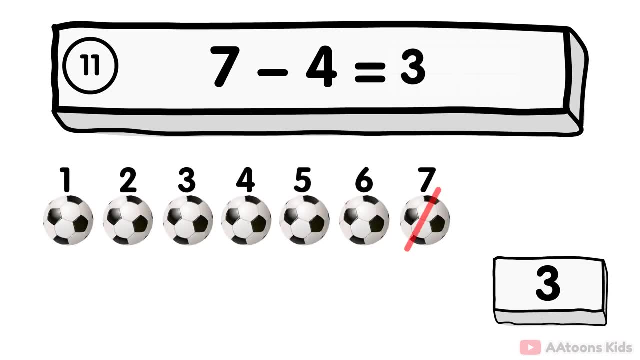 3 multiplied by 8 is equal to 6.. 1 multiplied by 9 is equal to 5.. Let's take the biggest number, 7, and subtract 4 from 7,, 1,, 2,, 3,, 4.. 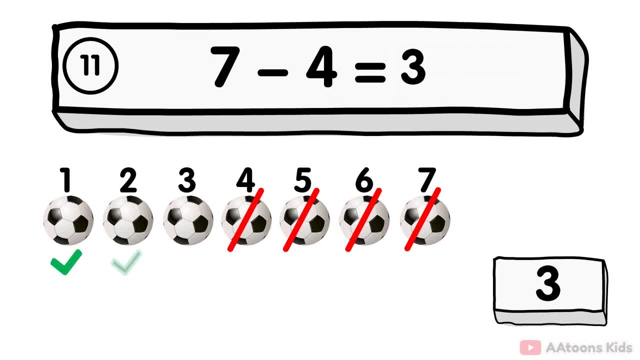 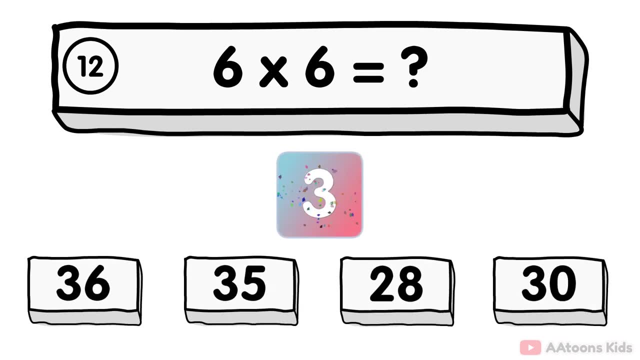 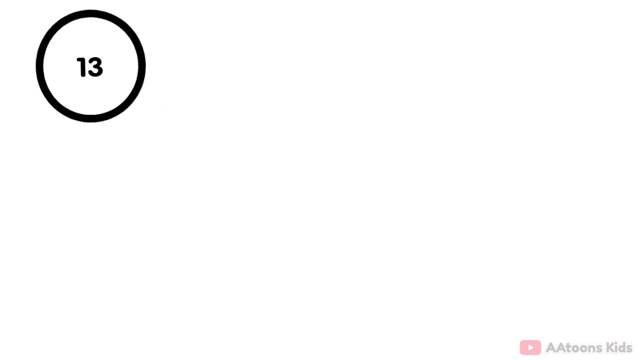 Now count the remaining balls: 1,, 2,, 3.. So 7 minus 4 is 3.. 6 multiplied by 6 is equal to 36.. 6 multiplied by 6 is 36.. 6 plus 3 is equal to 36.. 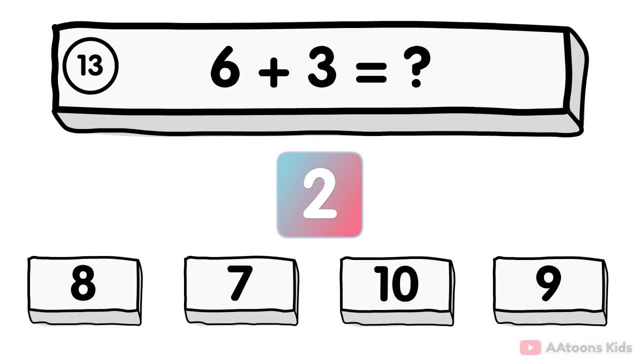 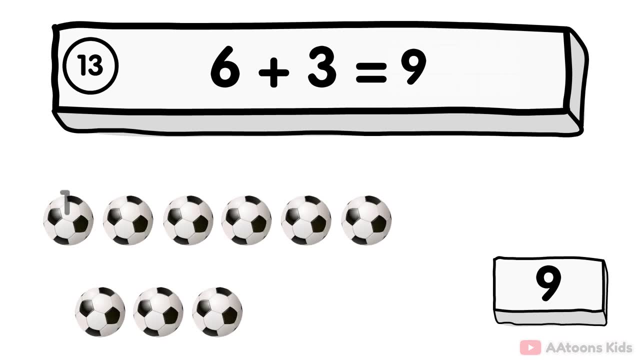 36. 9.. Let's take 6 balls and 3 balls. Now count together 1,, 2,, 3,, 4,, 5,, 6,, 7,, 8,, 9.. 5 multiplied by 6 is 36.. 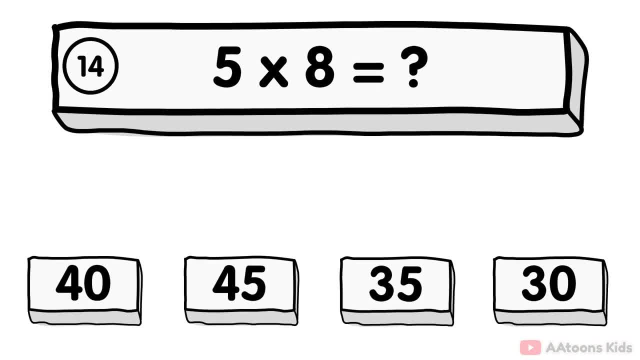 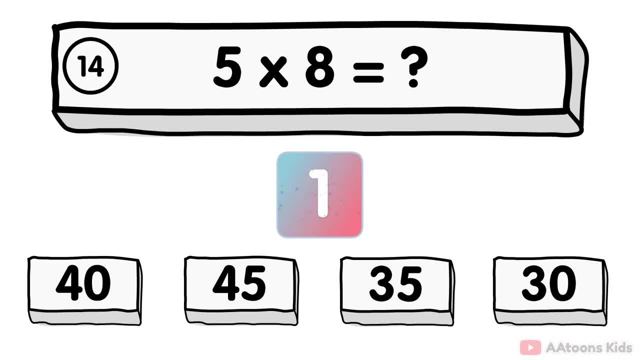 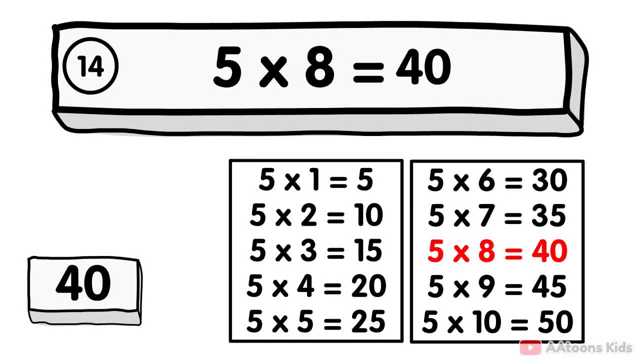 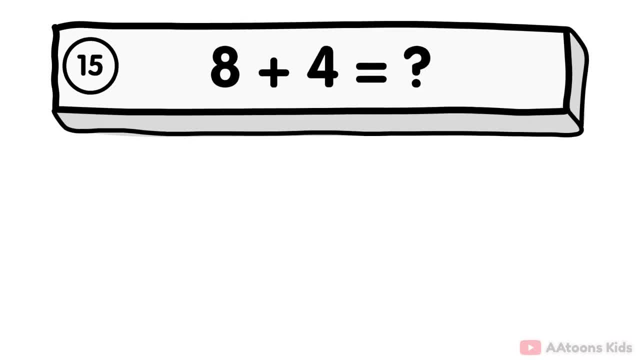 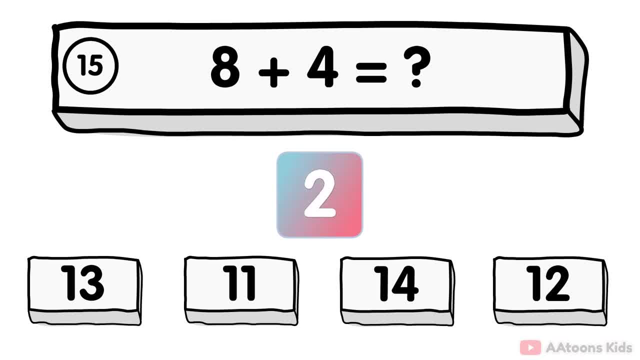 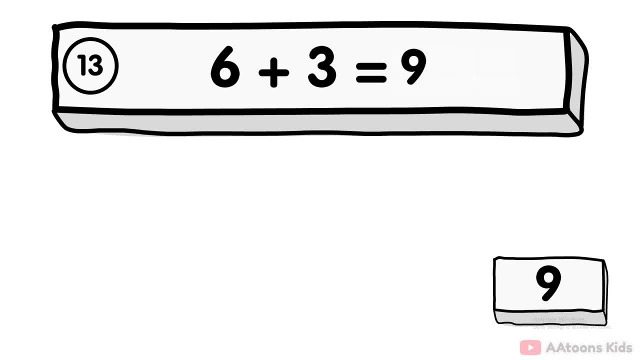 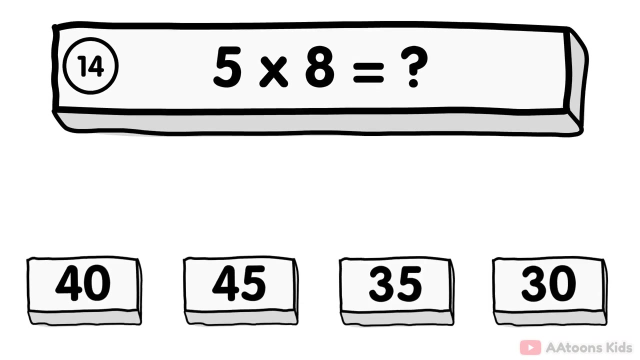 9.. Let's take 6 balls and 3 balls. Now count together: 1,, 2,, 3,, 4,, 5,, 6,, 7,, 8,, 9.. 5 multiplied by 8 is equal to: 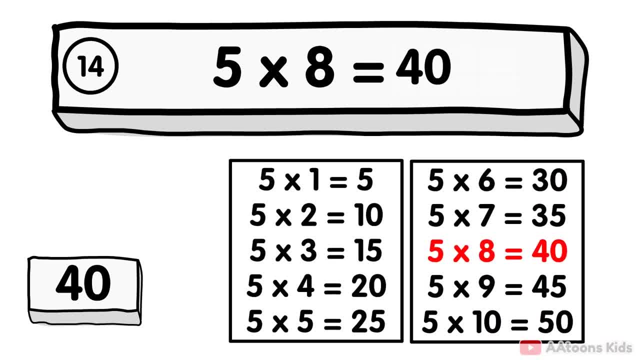 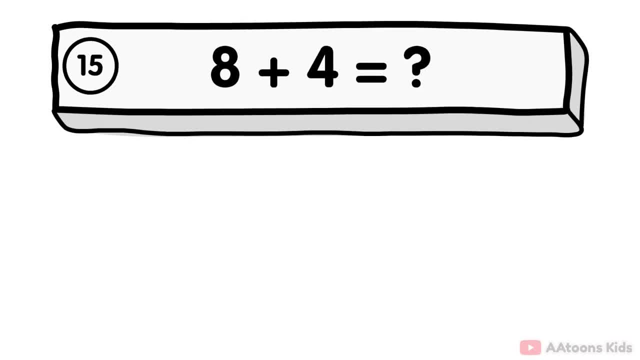 40.. 5 multiplied by 8 is 40.. 8 plus 4 is equal to 2.. 1,, 2,, 3, 4 is� 60.. 4 plus 8 is нажmwe. 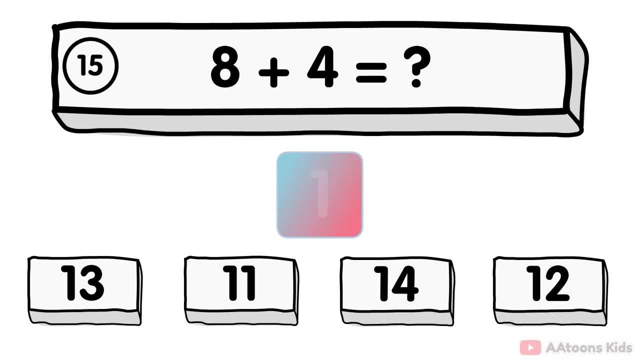 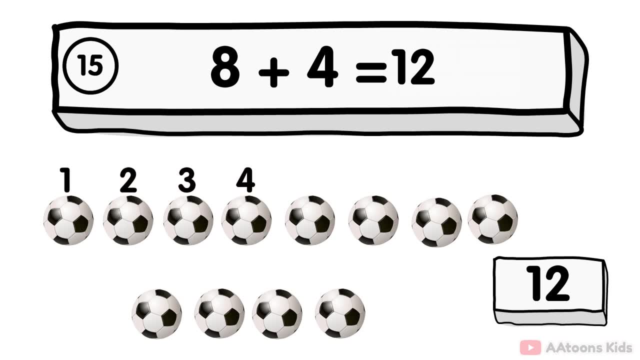 32. 60. 2,, 2, 3,, 4 is 60.. 80. Let's take 8 balls and 4 balls. Now count together 1,2,3,4,5,6,7,8,9,10,11,12. 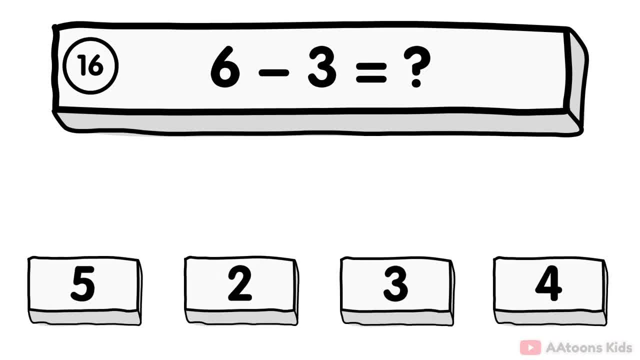 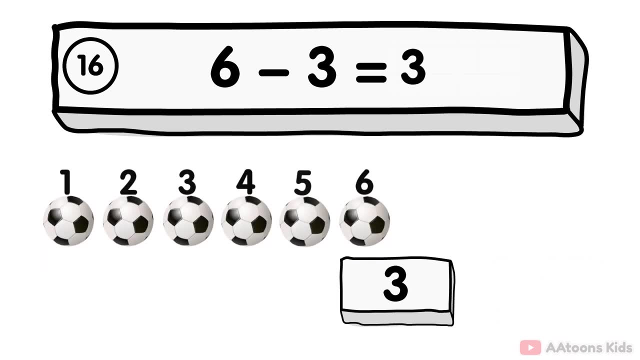 6-3 is equal to 3.. Let's take the biggest number, 6, and subtract 3 from 6.. 1,2,3.. Now count the remaining balls: 1,2,3.. So 6-3 is equal to 3.. 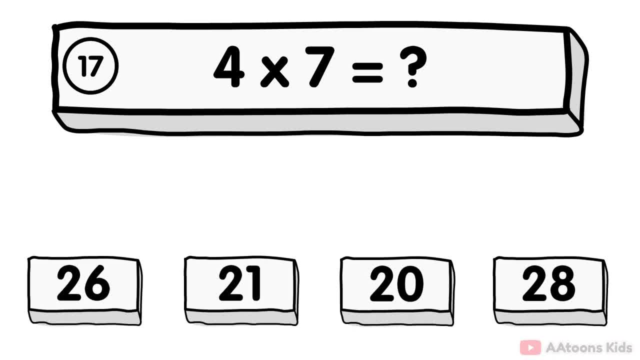 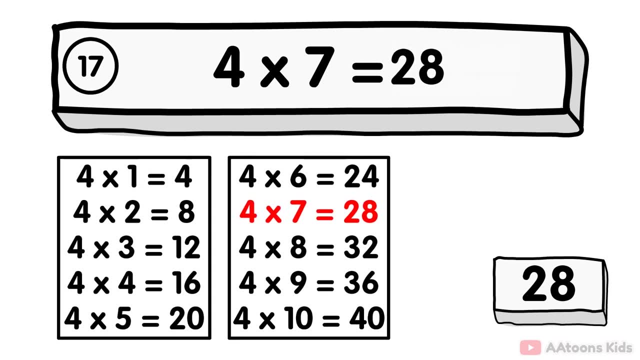 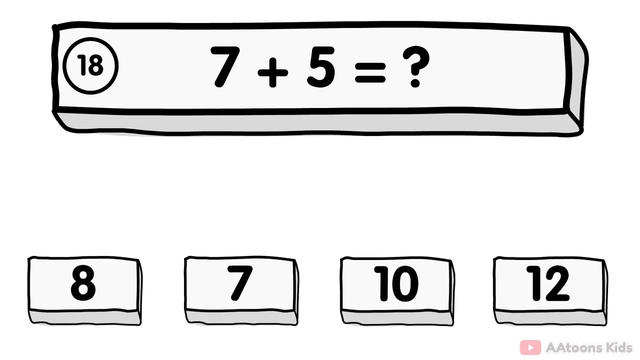 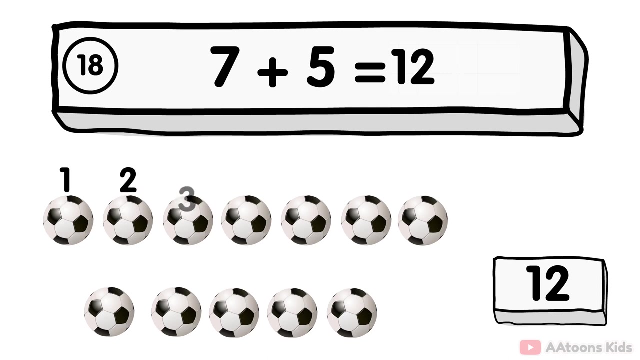 4 multiplied by 7 is equal to 28.. 4 multiplied by 7 is equal to 28.. 7 plus 5 is equal to 12.. Let's take 7 balls and 5 balls. Now count together 1,2,3,4,5,6,7,8,9,10,11,12. 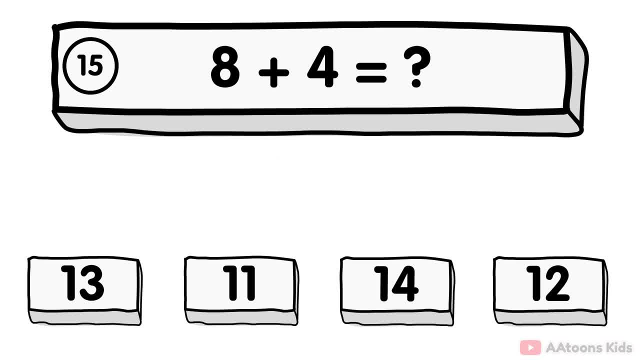 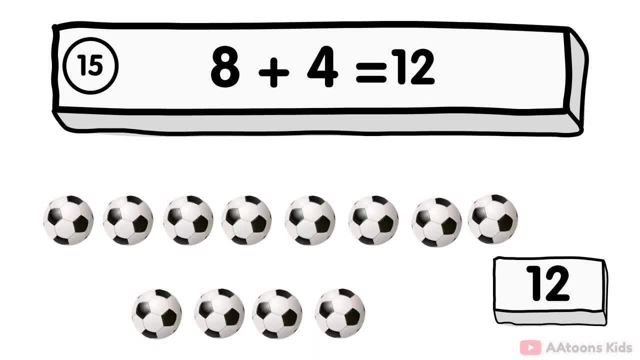 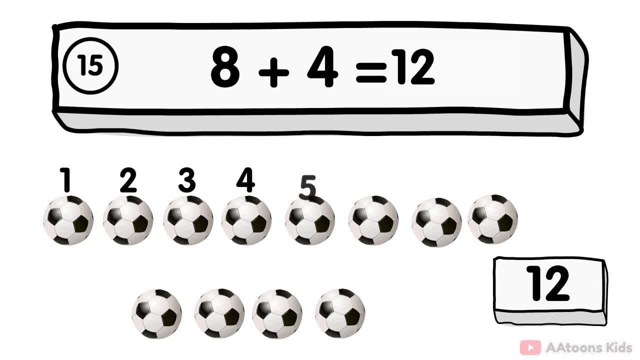 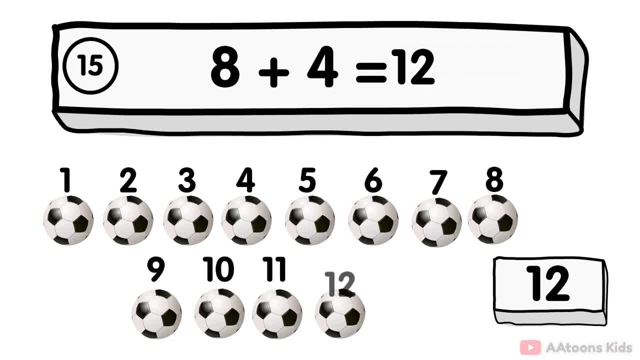 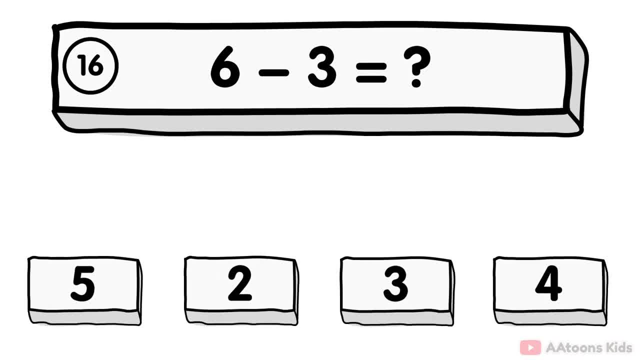 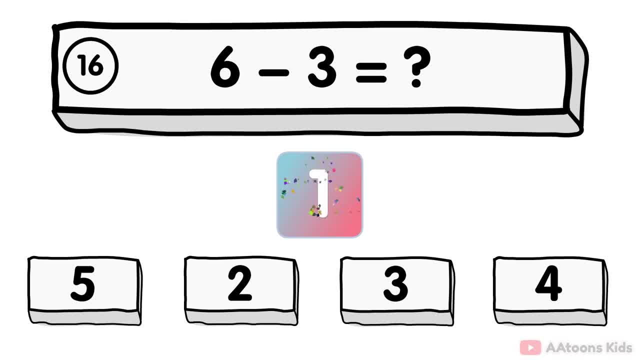 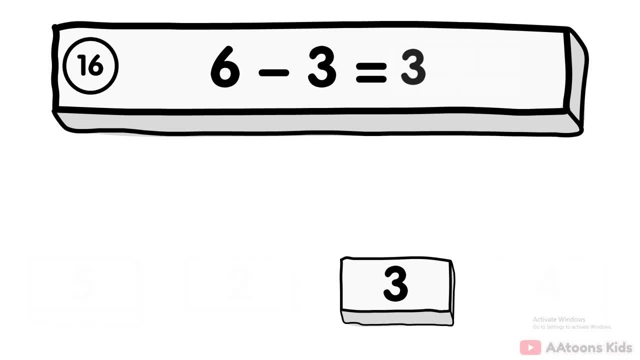 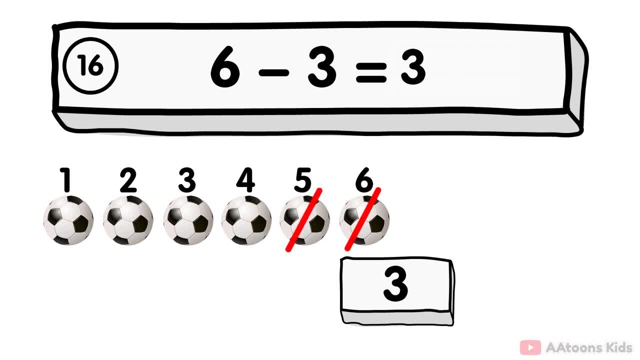 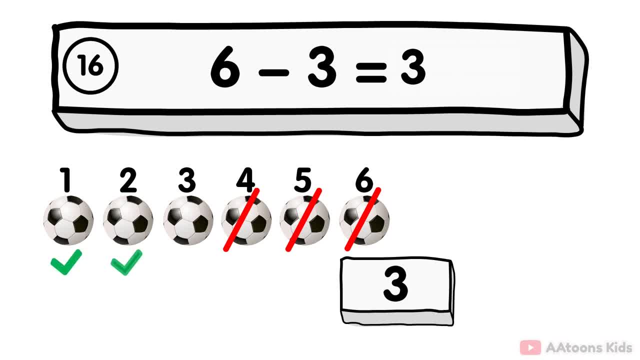 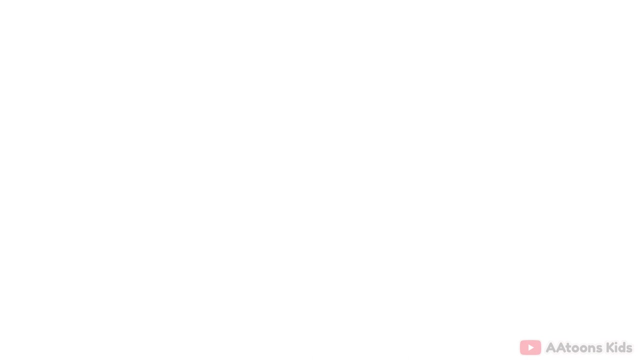 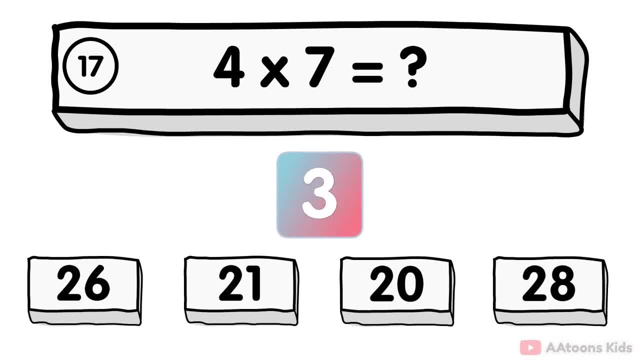 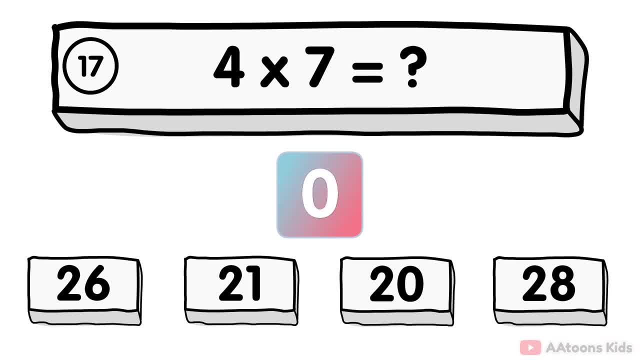 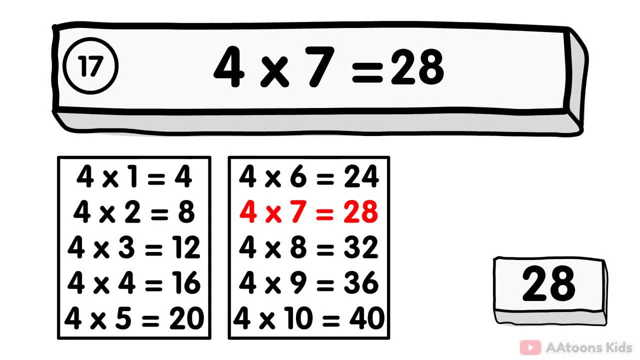 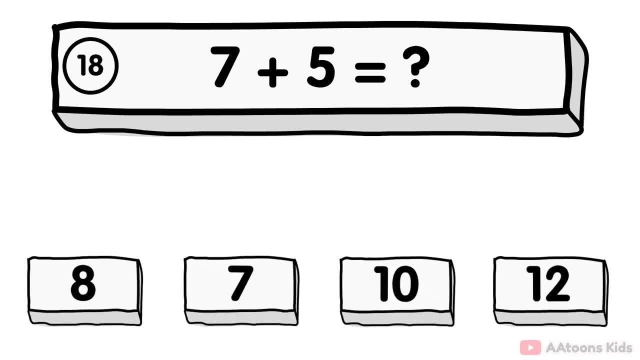 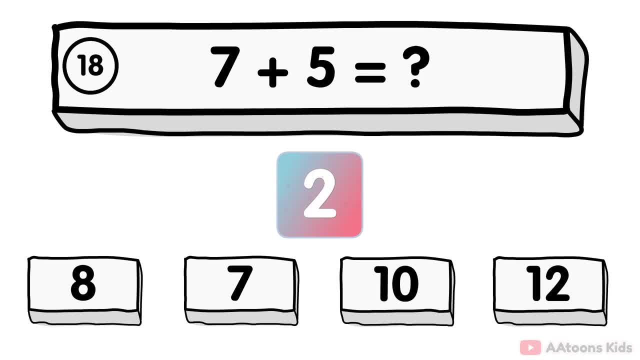 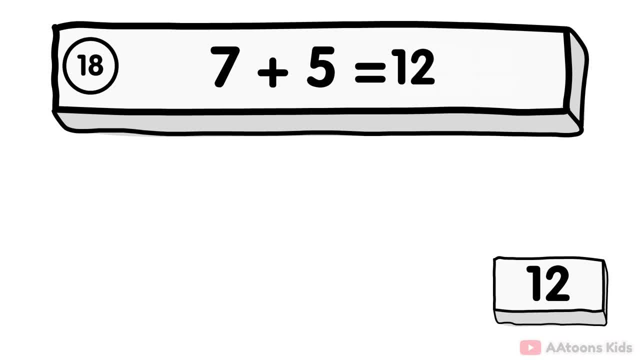